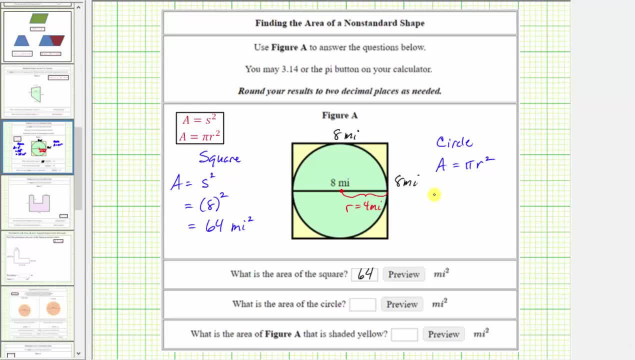 four miles, which means the area of the circle is equal to pi times the square of four miles. Four squared is equal to 16.. Pi times 16 is equal to 16 pi, And the units again are square miles. So this is the exact area of the square. 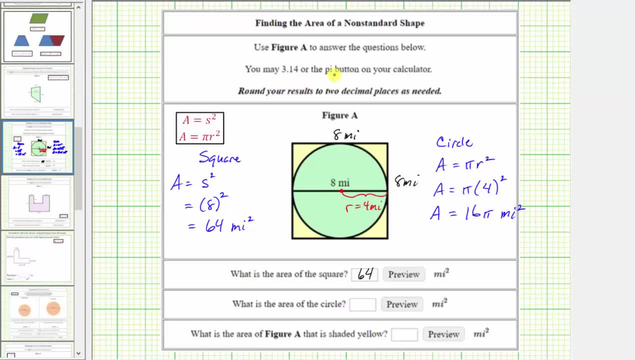 But for this question we are told to use 3.14 or a pi button on the calculator and then round to two decimal places. Well, we'll use the calculator to get a decimal approximation for the area We enter 16.. 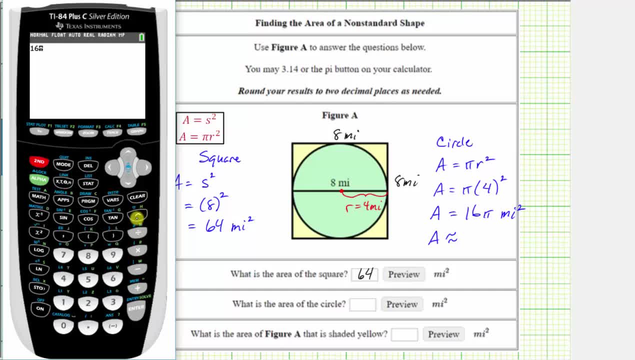 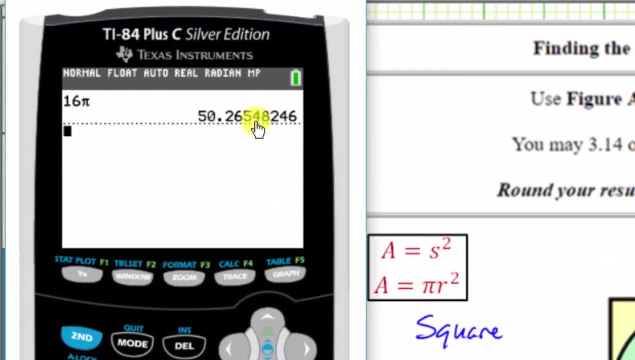 On this calculator the pi key is second and then the exponent key or the caret enter. We are rounding to two decimal places. So notice how we have a five in the thousandths place value, which means you round up. This is approximately 50.27.. 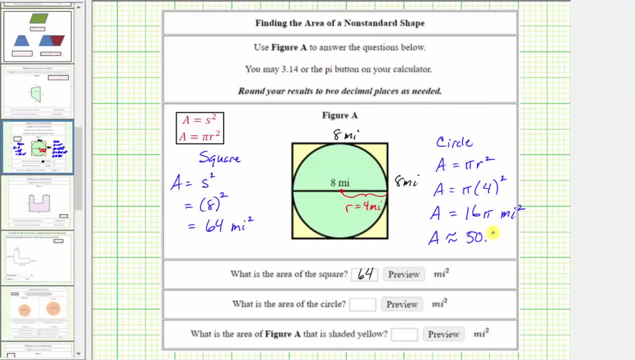 And therefore the area of the circle is approximately 50.27.. 50.27 square miles. We enter 50.27 below. the units are already here, But I'm also going to write down the exact area here on the right, which is 16 pi square miles. 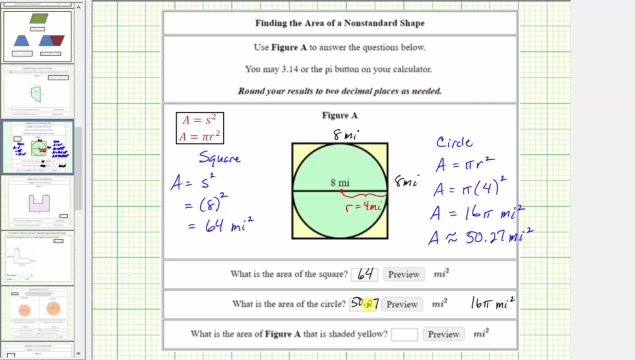 And now for the last part of the question. we're asked to find the area of the yellow shaded region, which again is the area inside the square but outside the circle, Or we can say the area between the square and the circle. 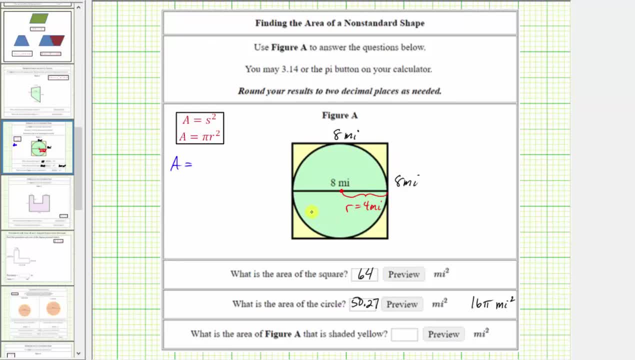 To find the yellow area, we will take the area which is the area inside the square but outside the circle, Or we can say the area between the square and the circle. To find the yellow area, we will take the area which is the area of the square. 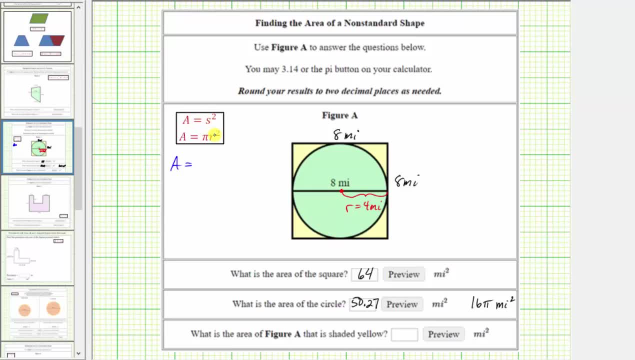 and subtract the area of the circle Using the area of formulas, this would be s squared minus pi r squared, And we already know these areas: The area of the yellow shaded region, or the area inside the square and outside the circle, or the area between the square and the circle. 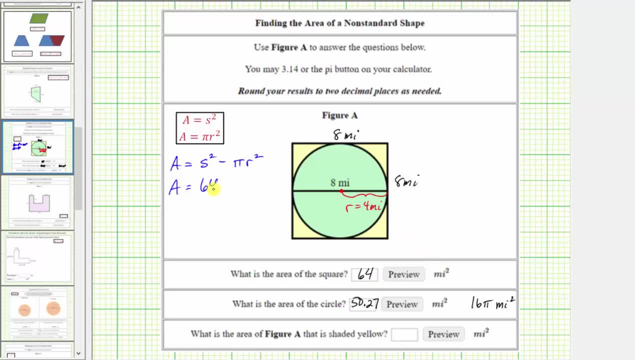 is equal to 64 square miles minus 16 pi square miles, and we know 16 pi is approximately 50.27.. We'll say the yellow area is approximately 64 minus 50.27, which is equal to 13.73,.